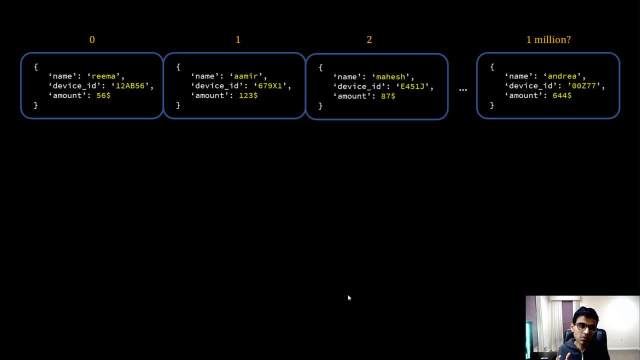 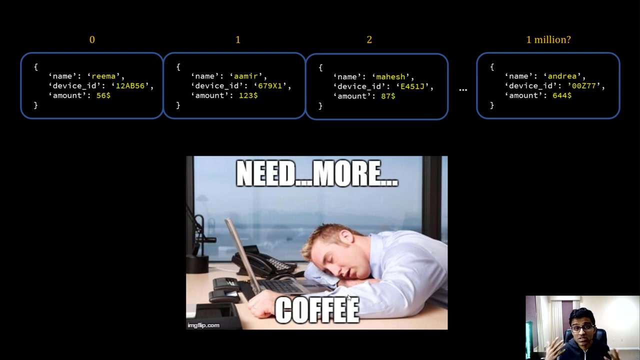 Linear search is not very efficient because just just think about if you have 1 million transactions. In that case, if you are looking at the very last element, you are just performing iterations 1 million times. You need some coffee. It's so much tiring work even for 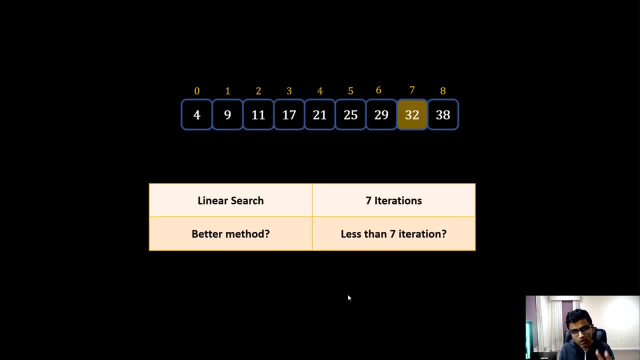 a computer. Going back to our numbers, example, linear search took 7 iteration to find number 30. think about any better method which can do the same task in less than seven. actually, you can pause the video and you can just do some thinking on this problem and you will be able to find the 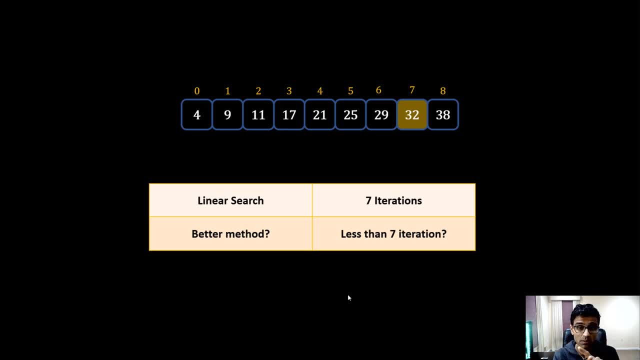 solution, because there is no rocket science. one thing you need to remember is the list is sorted okay. so binary search works on the concept of sorted list. so in the sorted list, how do you find 32 in a way so that you don't have to perform seven iteration? all right, that technique. 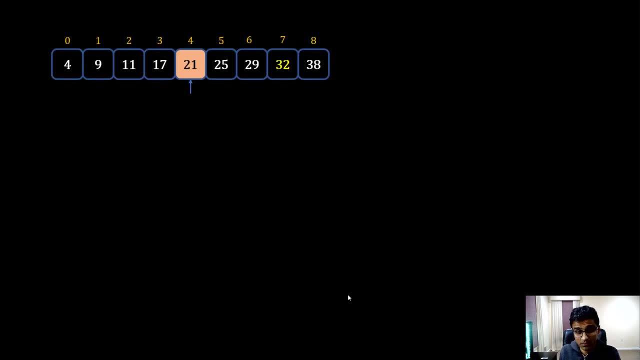 is this. so you take the middle element, which is 21, you compare it with 32. of course it is less than 32. now, by doing this comparison, you have ruled out the possibility that the number exists in the left hand side of this array. so all the elements from 4 to 21 which I have, 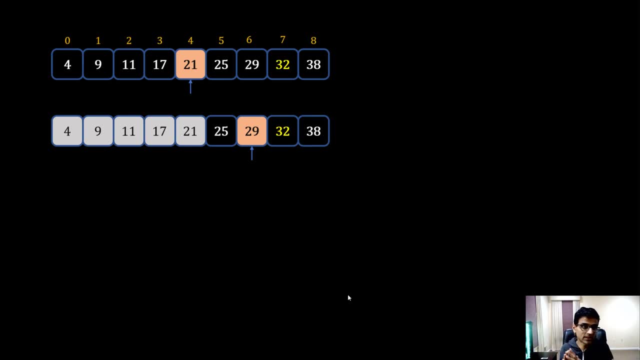 grayed out here. you know that the number is not in that particular portion of the array, so you can discard it. so see, in the first comparison is itself: you discarded half the elements. now you go to the middle of the remaining array. I have an array of size 4 now, 25 to 28, those last. 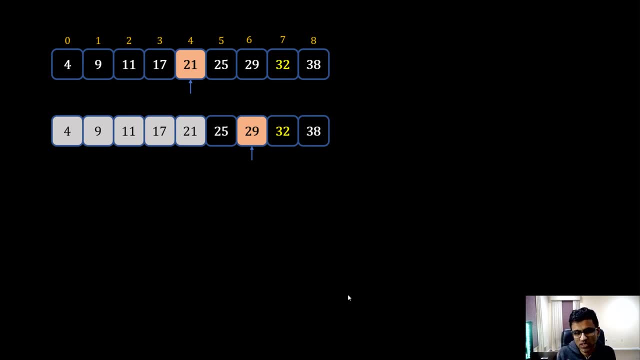 four elements, the middle. you can say it's 29 or 32, but let's go with 29, and then you compare. you don't find 32 here again. so then you again discard that left hand side of array, which is 25 and 29. now you are left with only two elements: 32 and 38. and when you take a middle, well, 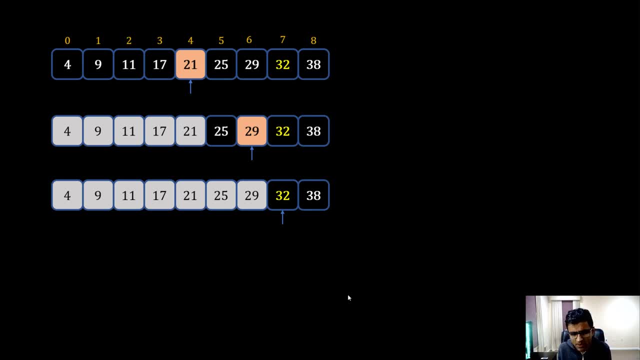 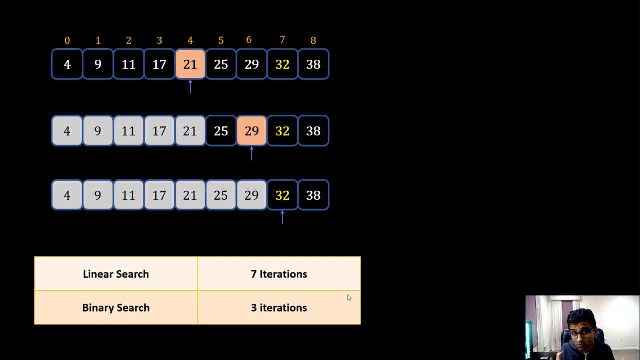 middle of 32, 38 is either 32 or 38, doesn't matter. and now you can do this operation in three iterations. so this is called binary search. in binary search, in every iteration you are dividing your search space by half. so iteration one: you discarded n by 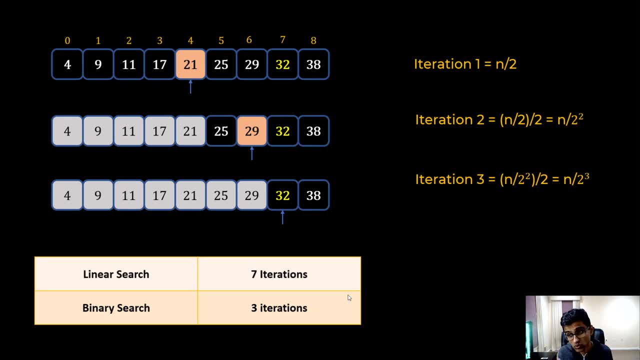 two elements. in iteration two it is n by 2 raised to 2, because again you are doing n by 2 divided by 2. okay, I think it's so simple math. you get an idea. in iteration k it will be n divided by 2 raised to k. 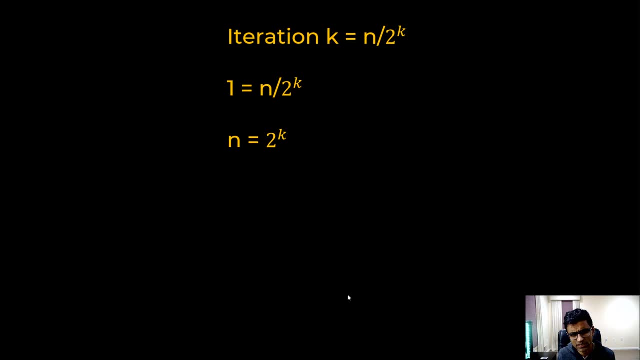 so, going over this math a little bit more in detail, you can normalize this equation and say: n is equal to 2 raised to k. this is simple mathematics. if you put log in front of both left and right hand side of equation, you get this, and then on the right hand side, k, of course you. 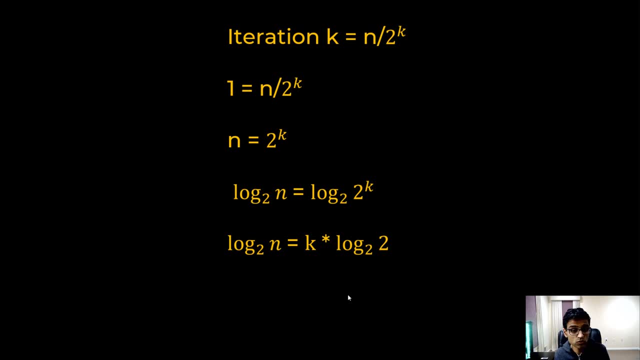 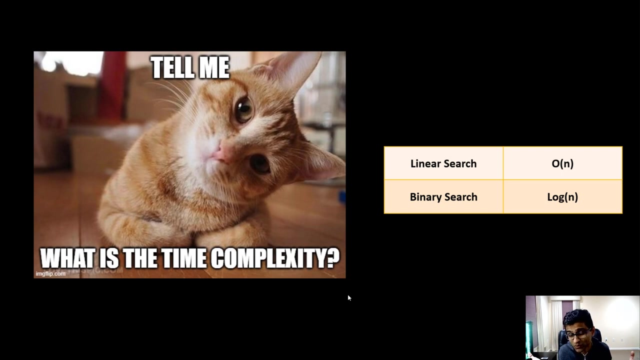 can take in the front. so you get this now. log 2 to the base 2 is actually 1.. so let's make that one to log n. so the search, the time complexity for binary search is order of log n. so now you just answer the question of this curious cat, which is: what is the time complexity? well, linear search is. 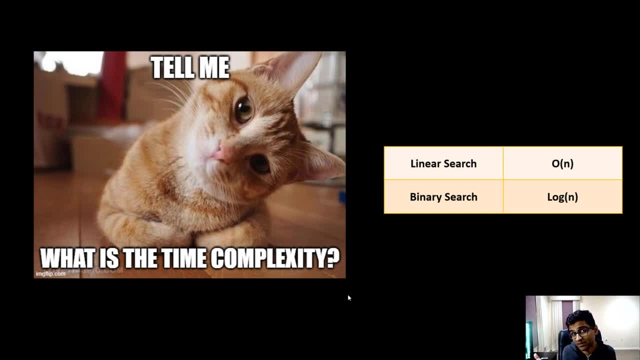 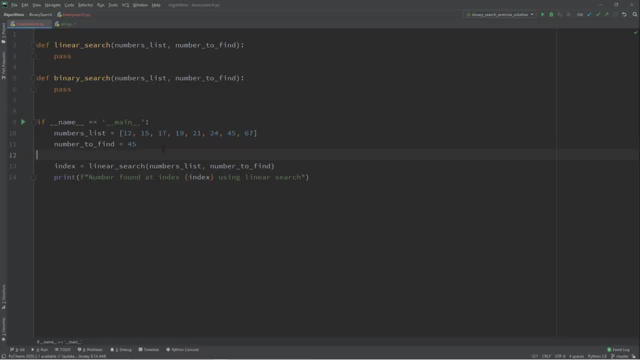 order of n. binary search is: log of n. let's implement binary search in python. now. I have this code written in my pycharm where I have a list of numbers. I want to find number 45 from that, and first I will find it using linear search. linear search is: 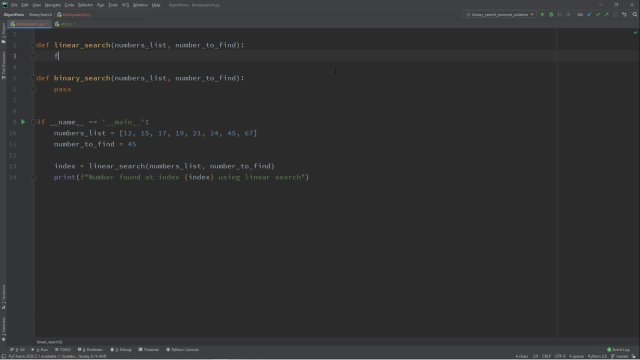 just running a simple for loop on these numbers. in python you can write something like for index element in enumerate. so when you have a list and when you call enumerate, it will return you index as well as an element and whenever element is equal to number to find. 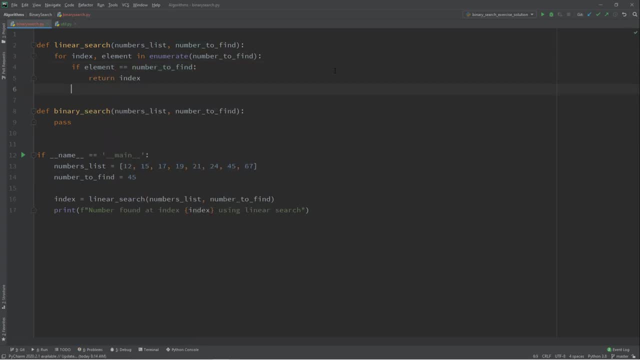 you can return that index back, and if it is not found, the general convention is to return minus one. if you right click and run this code here, it says: object is not iterable because let's see the here. I should have number list and if I is at index six, one, two, three, four, five and six, if you type in, let's say big number which, 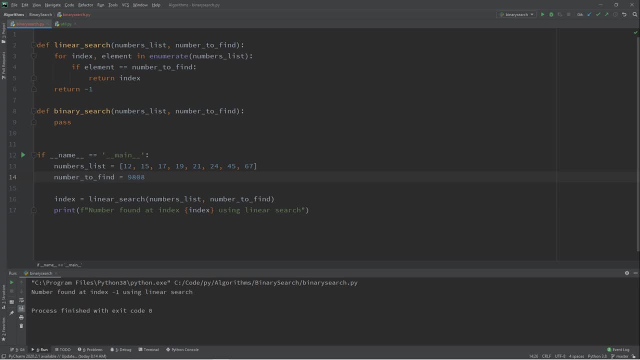 is not in the list, it will return you minus one. so linear search works. okay. I want to now do the same thing using a binary search, so let's change this to binary search and this is a binary search, and in binary search. now what we are going to do is the technique that we saw in a presentation, which is we 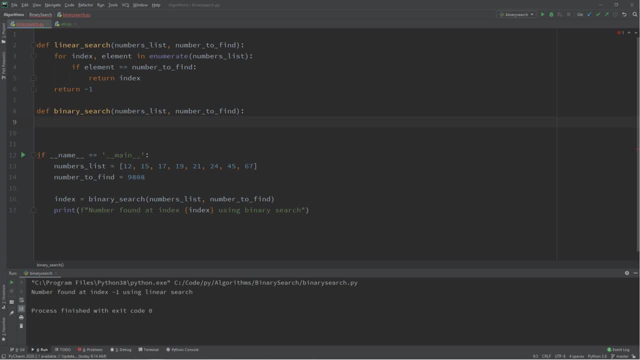 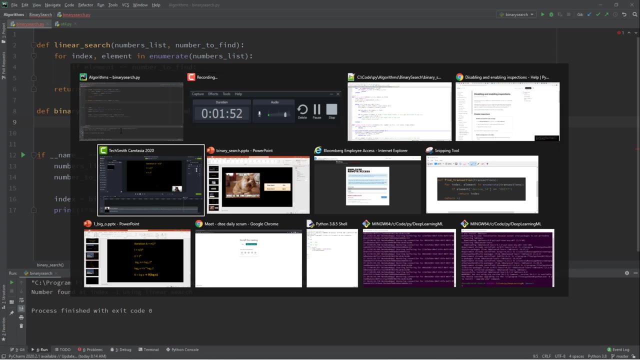 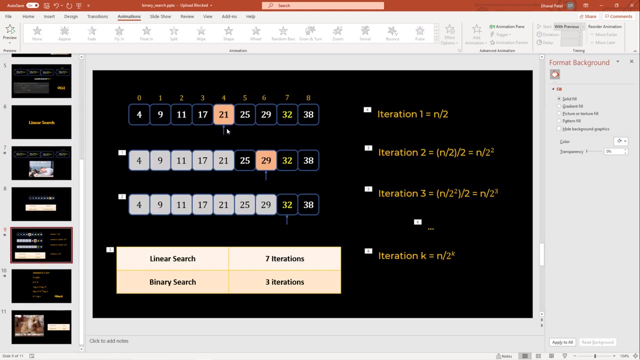 will look at the middle element first. okay, so let's call the left partition and right partition. so we are almost doing like left and right partition here. so if you look at this thing, uh, here we looked at the middle element and then we eliminated all the array elements in the left. 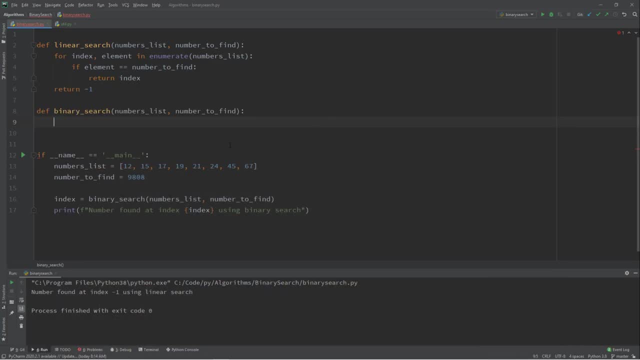 side. okay, so there is this concept of left partition, right partition, so I will use left index is equal to zero. okay, right index. let's set it to the last element, which is length of numbers list minus one or a. I A starts with zero. that's why I'm doing minus one for the last element and let's say the. 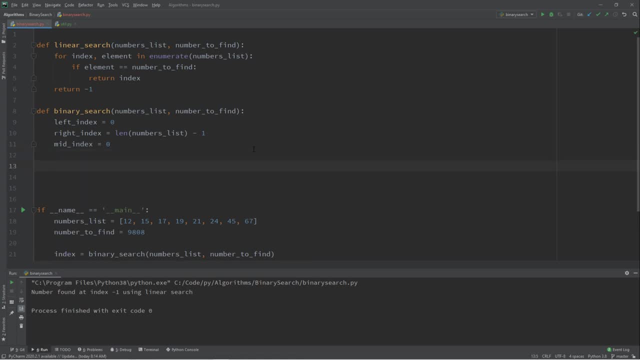 mid index for now is zero. now, mid index initially will be what foreign? it will be left index, okay, plus right index divided by two, okay. now in python, when you do divided by two, you have to use double two now. now, the way I verify all this is I go to terminal here. 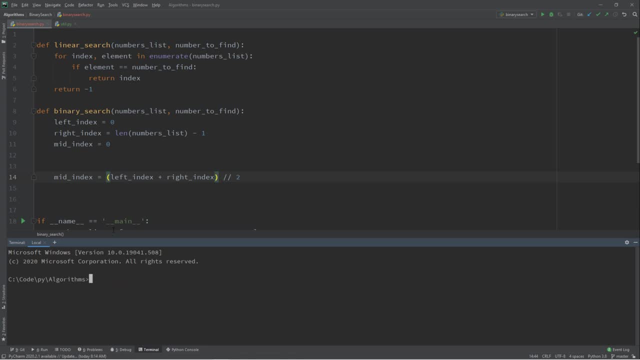 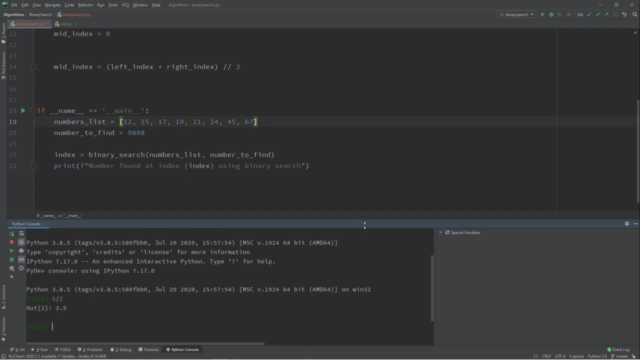 okay, this is my Python terminal and let's quickly okay Python console. so in the Python console, if I do, let's say, 5 by 2, you can see you are getting floating point number. when we want to get the middle index it has to be integer. so when you do 5 double slash 2, you get the integer portion and 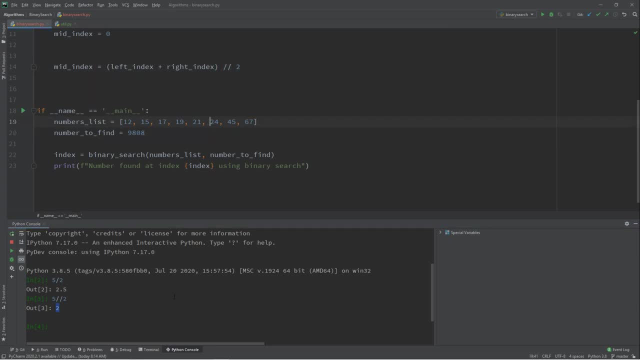 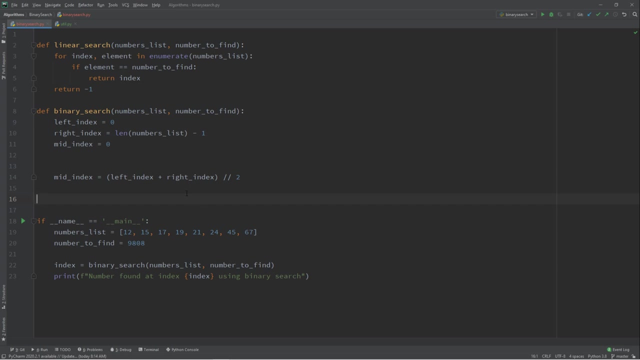 that is the reason I am doing double slash here. this Python console, or even you can run idle to quickly check a single line of code that you are not sure about. okay, all right, now, once you find a mid number, made index. you want to find a mid number, so my mid number is this right, and then you do comparison. now you will. 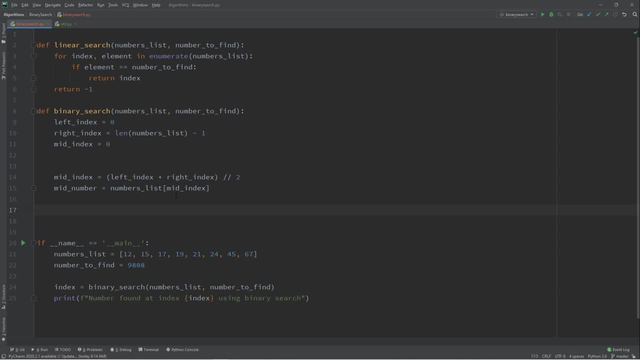 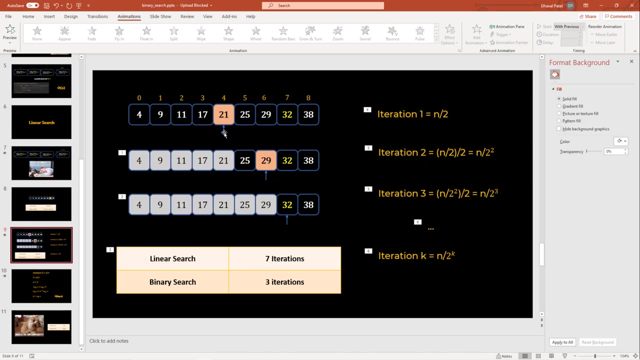 do all of this in a for loop, because you are doing this process repetitively and the for loop will look something like this: while left index is less than equal to right index, why we are doing that? well, here, this pointer that you are seeing is a mid index. 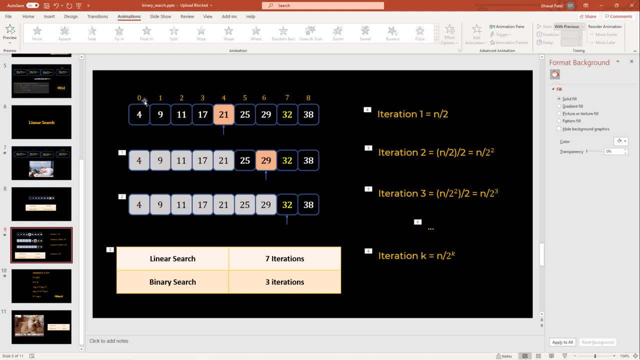 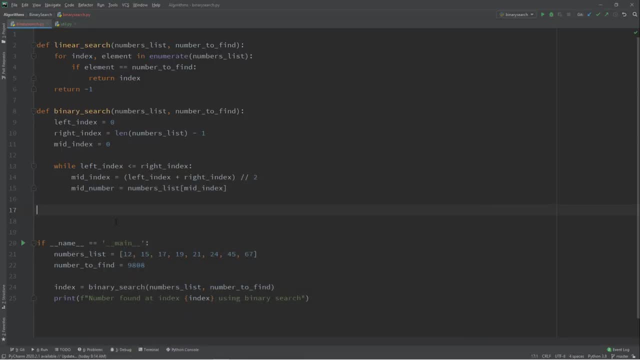 and every time. in the first iteration, my left index was 0, right index was 8. in the second iteration, my left index was 5. see, this is 5, right index is 8, and you keep on doing this until left index is less than equal to right index. okay, and 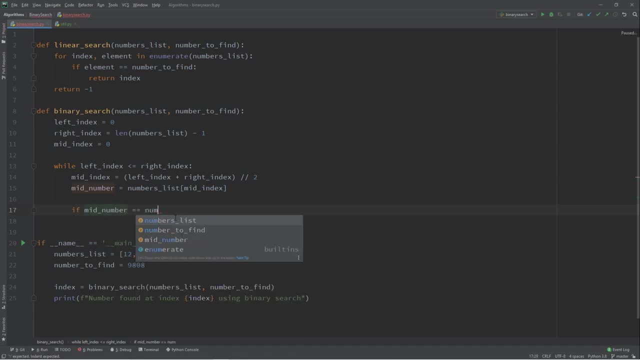 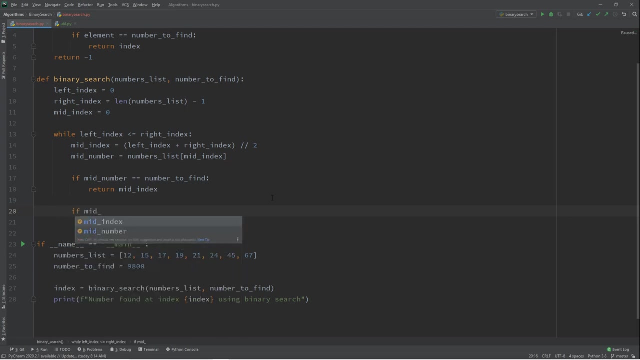 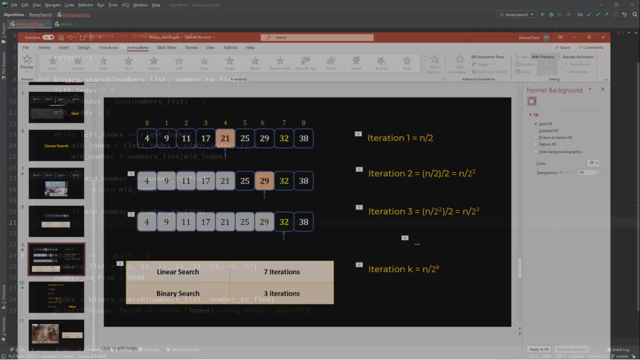 whenever the mid number is equal to number that you are finding, you can easily return that mid index, because that's the index you were looking for. but if it is not the that, and if mid number, let's say, is less than number to find, okay, so this mid number 21 is less than 32.. so in that case, what? 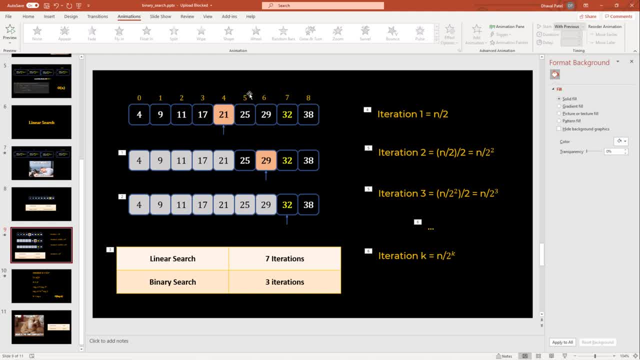 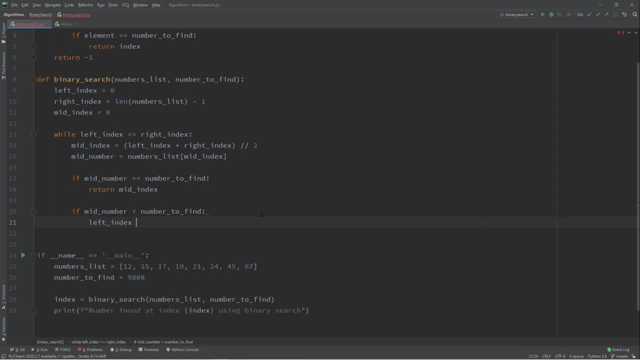 we do. we reset our left index from zero to five. so five is nothing but mid index plus one. so you are resetting your left index to mid index plus one and right index remains the same. so you will do: left index is equal to mid index plus one. okay, 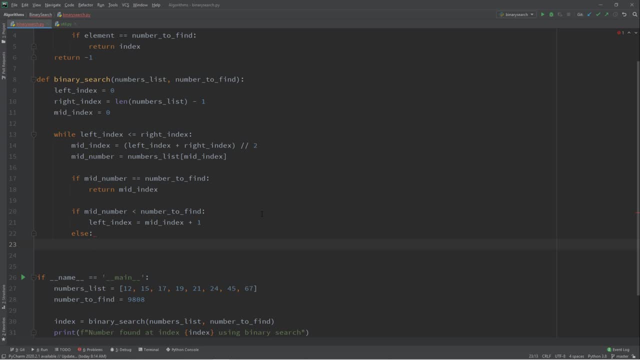 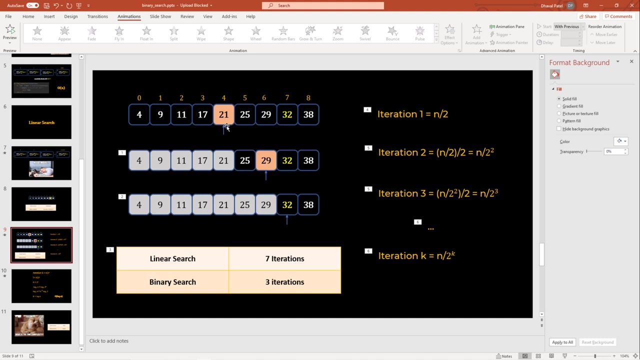 else else means mid number is greater than number to find, because took care of equal to case here. so the only possibility here is mid number is greater than number to find. so let's say here if we are searching for 9, then 21 is greater than 9. so then what you'll do is you will keep the left index as it is. 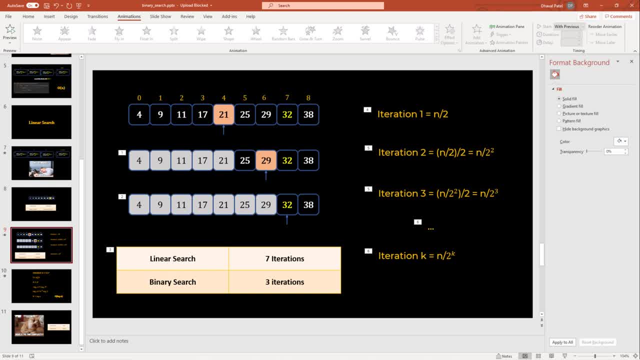 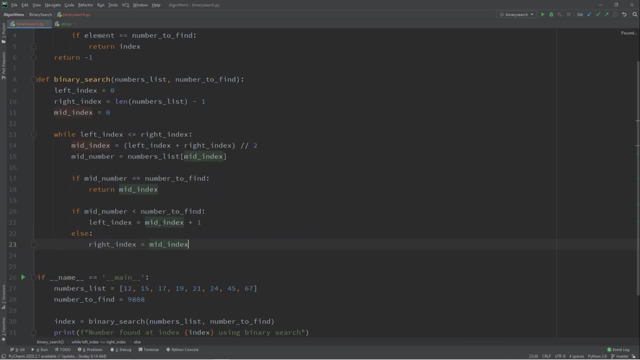 and then you will move your right index from 8 to number 3, because 21 you have looked at it and that 3 is nothing but mid index minus 1. so that's what we'll do here. so right index is made index minus 1. I hope it is making sense if you. 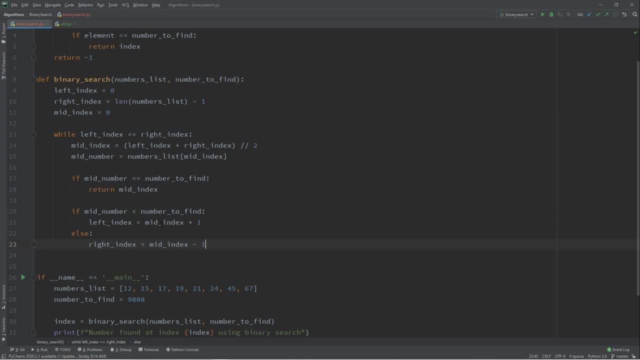 just pause this video, do little thinking. it is not hard at all, trust me, it is very, very straightforward. and then in the end, if you don't find anything, you return minus 1. all right, let's run this code now and see what happens. so we'll first run it. 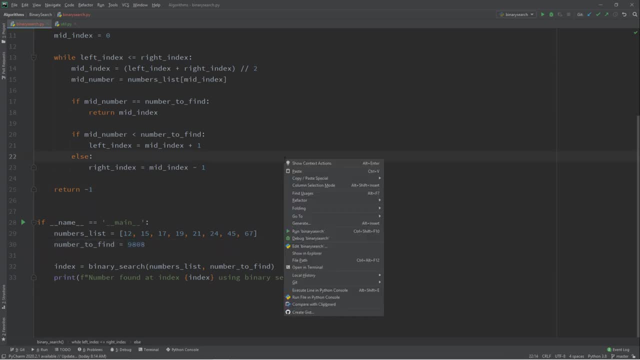 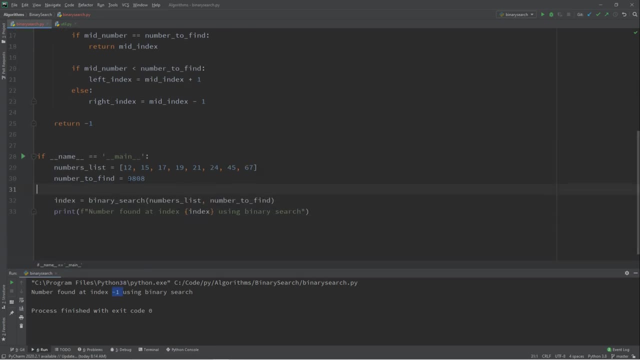 on a number that is not in the list. I am expecting minus 1 right-click run: see minus 1. now let's find 45, or maybe 24. see 24 is at number 5 right. 1, 2, 3, 4, 5. 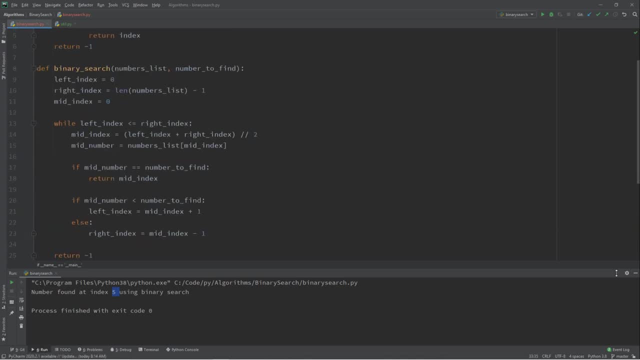 okay, I hope you enjoyed this video and I will see you in the next one. bye, bye. I always use debugging facility of pyjama to figure out what's going on, so for that you can set a breakpoint here, right-click debug, and when you do that, 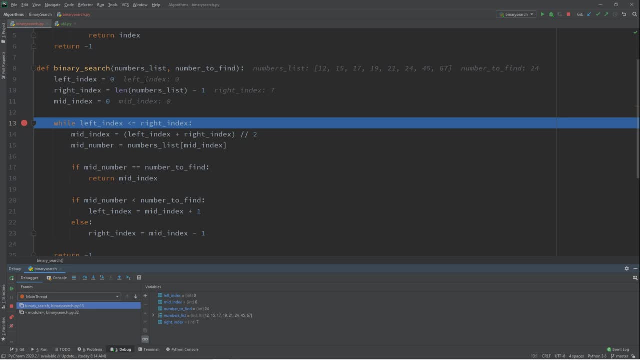 you can do a dry run. so here you see: left index is 0, right index is 7, and when you press on this button or this one, 1 by 1, see my mid index came out to be here you can see: mid index: 3. okay, and then you can do a dry run. so here you see. 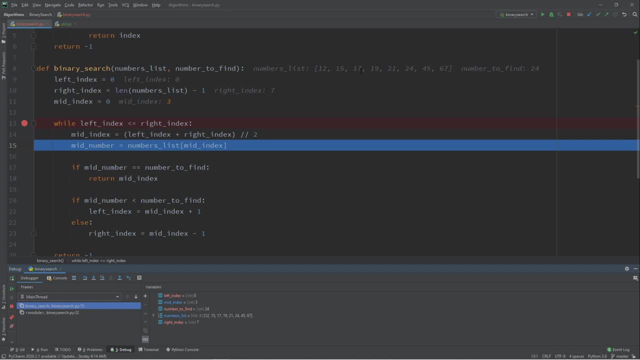 my mid index: 3 okay, so 0, 1, 2, 3. so 19 okay, and 0, 1, 2, 3 okay. and then my mid number is 19, all right, so mid number is 19. now, mid number is not what we are looking for. we are looking. 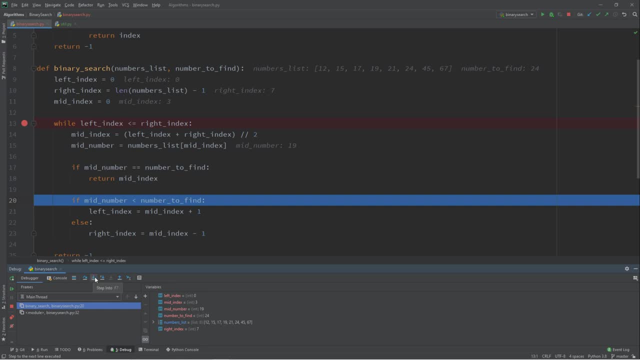 for 24. so then we will discard left inside of an array. so since mid number was less than number defined left index, we reset it to be 4. now, see, left index is 4 here. so now we got here at 21, okay, and then we take mid of that. so mid of that will be now 24, and 24 is the number we 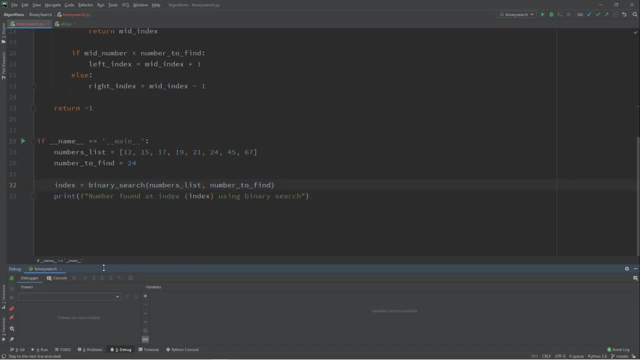 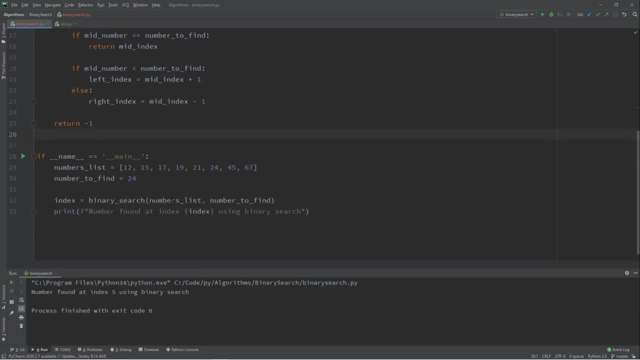 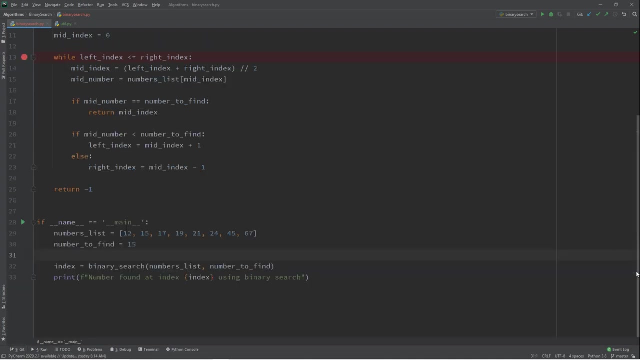 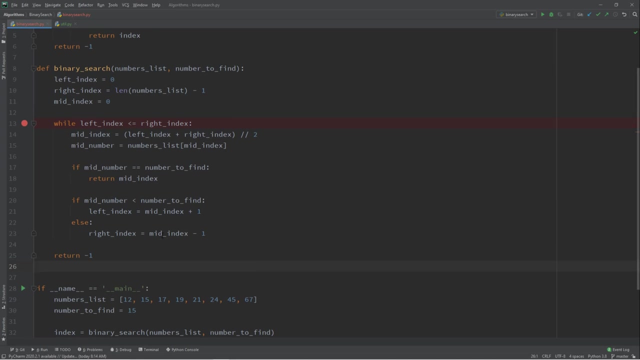 are looking for. so now we return it and we print it. so it is quite straightforward. okay, you can also look for different number less of 15, and it will find it okay. now we implemented binary search using a single while loop. you can also use a recursion because if you think about this problem, 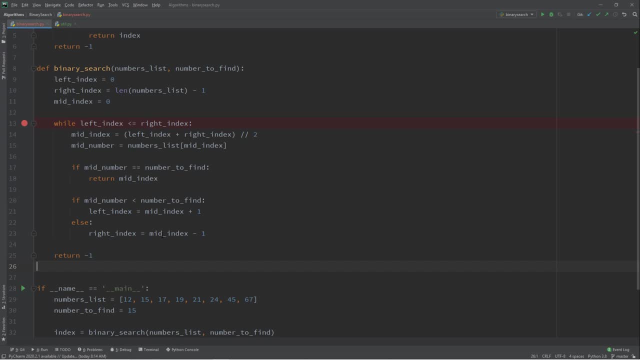 it's a recursive problem. at every point we are reducing array in half and on on that half array we are performing the same exit operation, and whenever you have this type of paradigm, you can use a recursion. so let's write binary search using a recursion now. so I'm going to do dev. 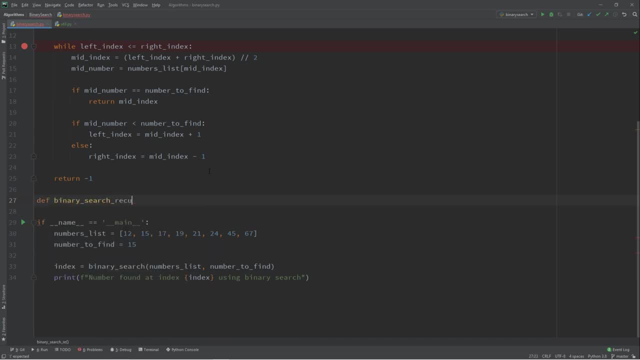 binary search recursive. before I do this, let's do one thing. I want to compare the performance of linear search with the binary search. how do I do that? or if you have seen my Python decorator video, which I'm going to link in the card as well as video description, below you can write a decorator like this: 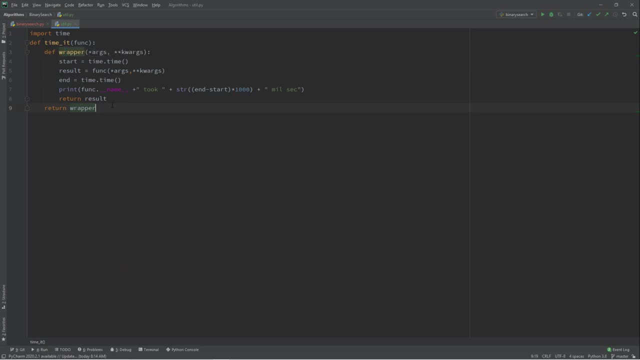 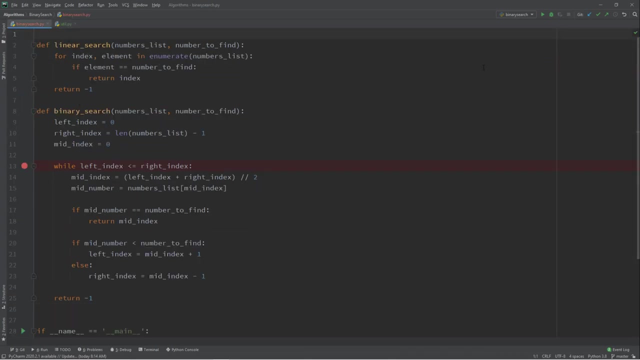 which will measure the time of the function. okay, so if you don't know about decorators, please watch that video. decorators are very powerful feature of Python. you should know it if you want to crack any Python interview here. in utilpy I wrote this decorator which I am going to import here in binary search. so from 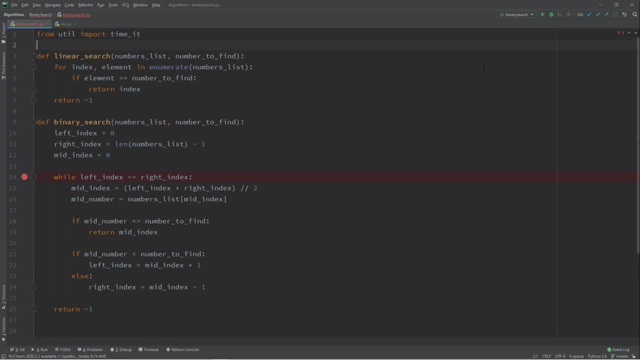 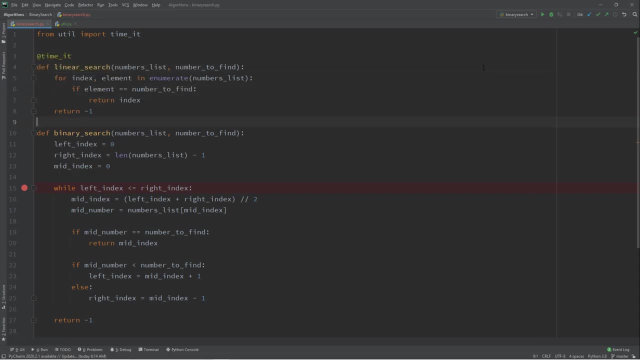 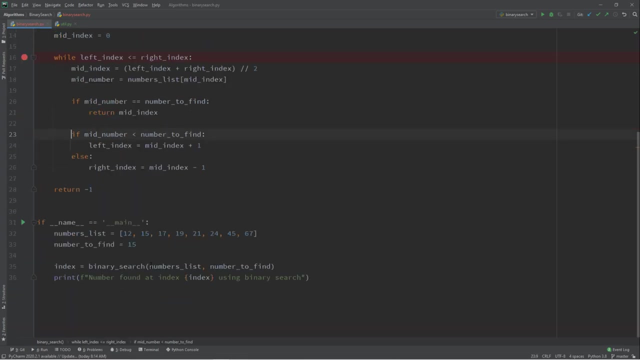 util import time. it okay, and I'm going to decorate this linear search as well as binary search, and when I do that, what will happen is now when I run this code. let's run it. it is also logging the time. it is saying binary search took 0.0. 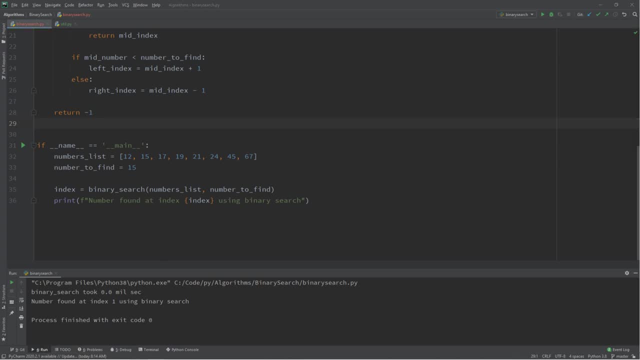 millisecond, because our array is very small. I want to make this array very big, okay, so let's make this array very big. so now my array has million element, million and one actually, and I want to find the last element. okay, and when you do that using, let's say first, let's do it using linear search. so 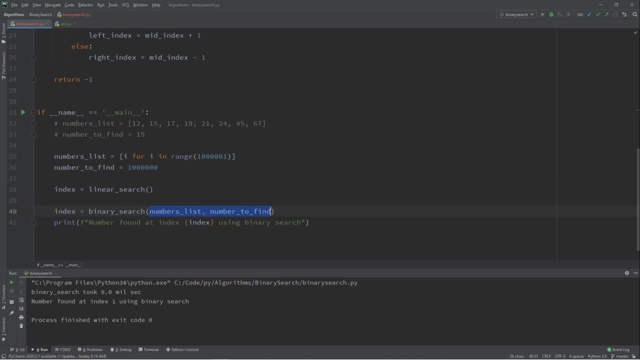 I'll do linear search and pass the same parameters. I will just comment this line because we know functionality wise, this works okay. so I'll just comment this line because we know functionality wise, this works okay. we are just measuring the performance. linear search took 31 millisecond, whereas binary search took almost 0. 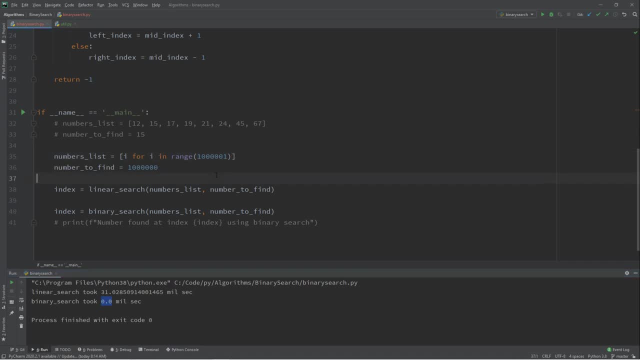 millisecond so you can see as number of element grows in the list. you can realize the benefit of binary search and in when you are writing big software programs you will be doing these kind of search operations very often. we looked at the case of electronic store tech. so we looked at the case of electronic store tech. 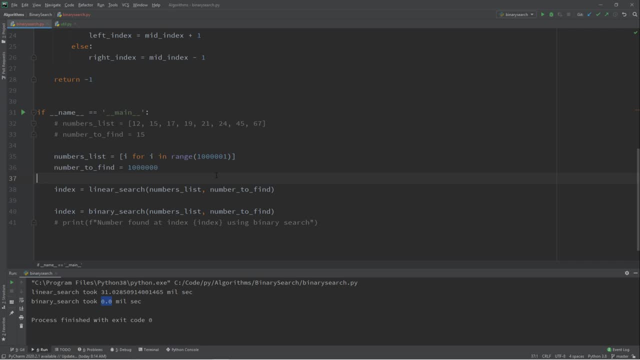 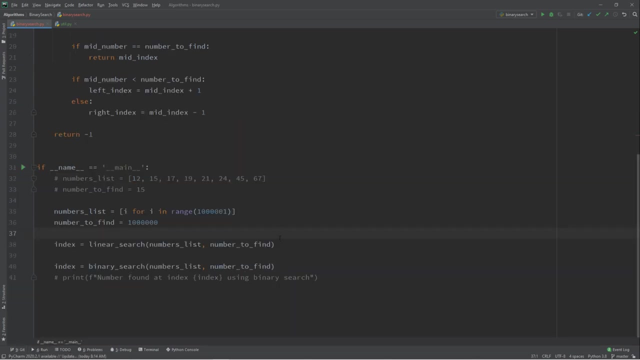 transactions, and for that reason, the knowledge of algorithms is very important, and you should be using efficient algorithm so that your overall program performance doesn't suffer. all right, we looked at performance now. now let's go back to our recursive way of binary search. so I define a new function. 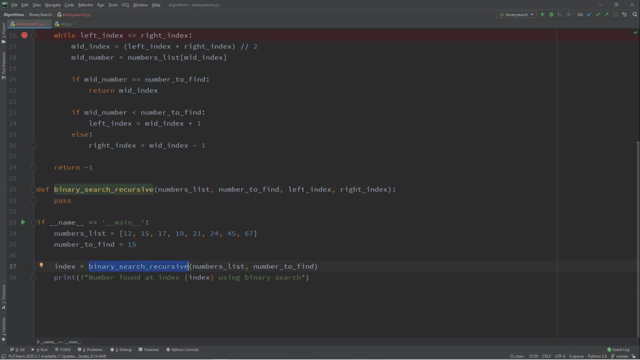 called binary search recursive, which I am calling it here. I added two more arguments called left index and right index, and we'll see why those are needed here. so think about binary search as a function which is taking the number list- left index, right index- and it is trying to find you the number in these. 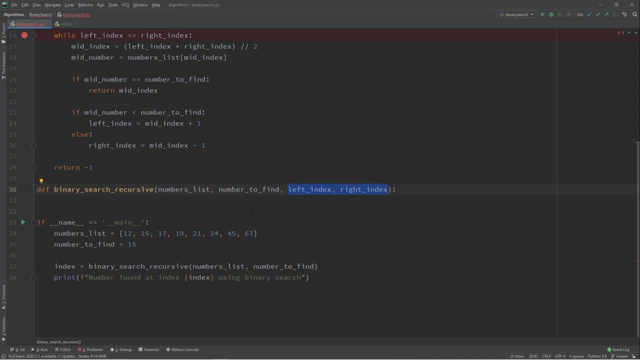 boundaries, okay. so if I say okay, 0 to, let's say, 3, it will. on, this function will only search for the number, which is the number, which is the number which is this much array. if I say 0, 1, 2, 3, let's say, 3 to 5, it will only search in this. 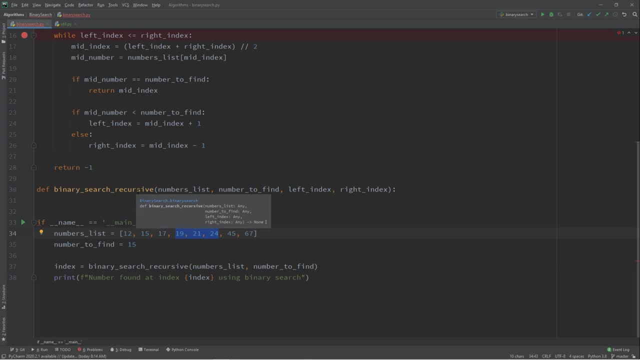 array. the role of this function is very simple: search this number in this left index and right index boundaries in this number list. okay, now, due to whatever reason, if right index is less than left index, then you want to return minus 1 minus 1, then you want to return minus 1, then you want to return minus 1 minus 1. 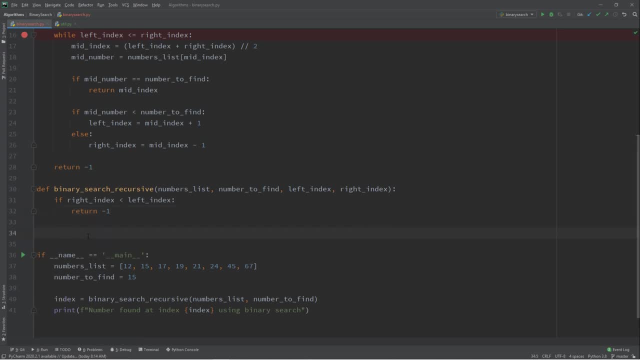 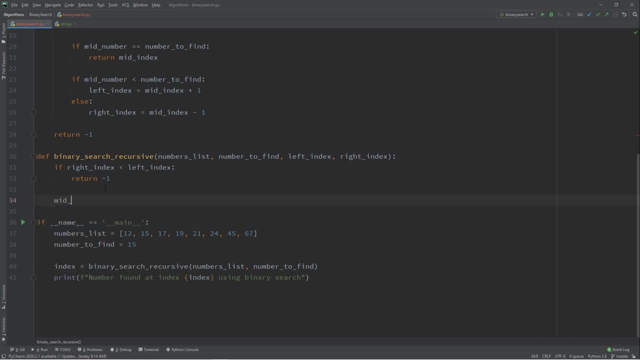 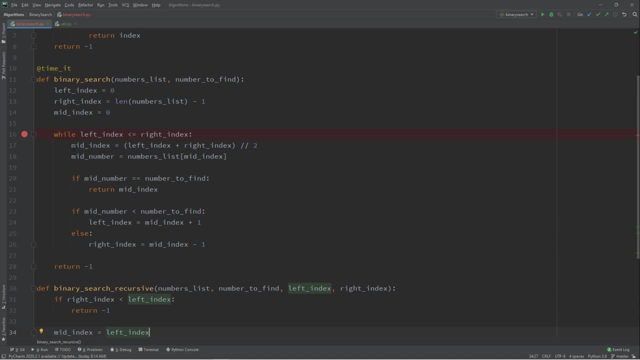 1 is a standard number that we return when we don't find the element. so right index has to be greater than left. if it is not, I am returning minus 1. then you find mid index, which is, which is same as what we saw here. okay, so mid index is: 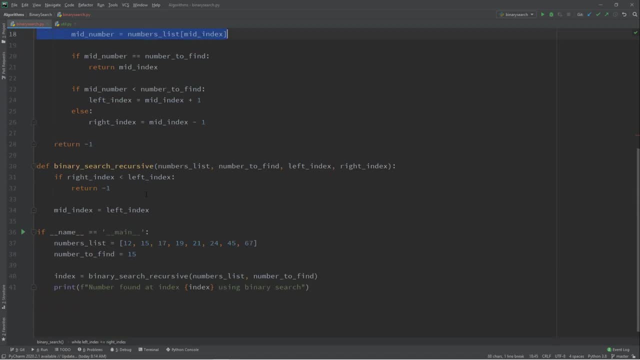 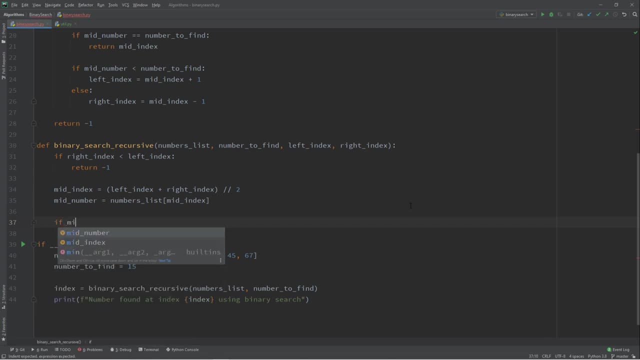 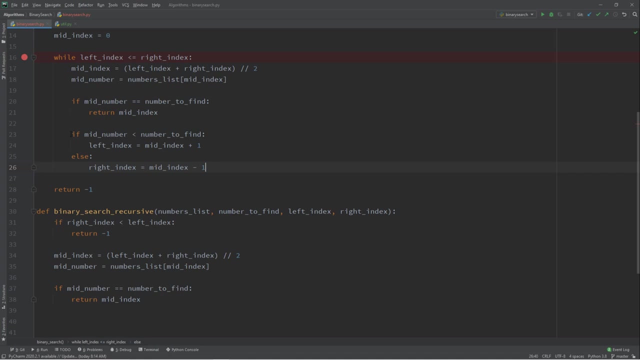 nothing. mid index and mid number are the same thing that we saw in regular binary search function, and if mid number is less than left index, then we return. minus 1 is the number you are looking for, then of course return the main index. so we're kind of writing the same code here. okay, so we can just copy paste this. 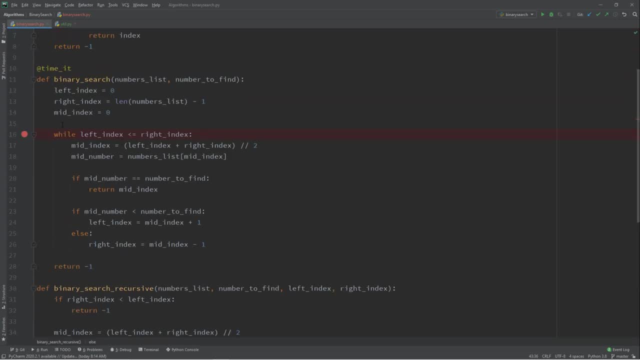 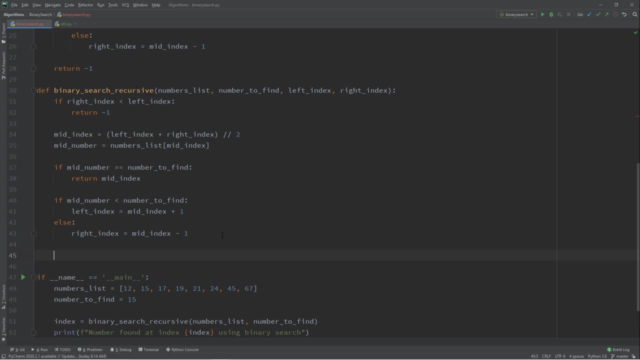 essentially these two functions are same. it's just that here you are doing it using while loop, here you are using recursion in recursion. you don't have loops. so when you find this new one in recursion in recursion, you want to find this new one in recursion. so we are going to write a function like this. so 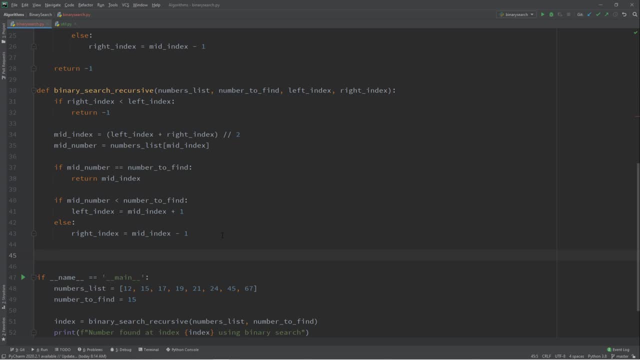 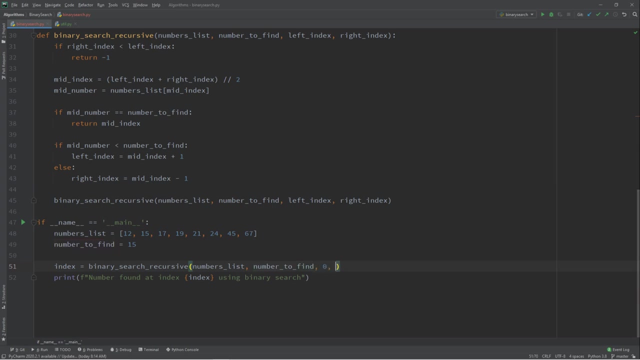 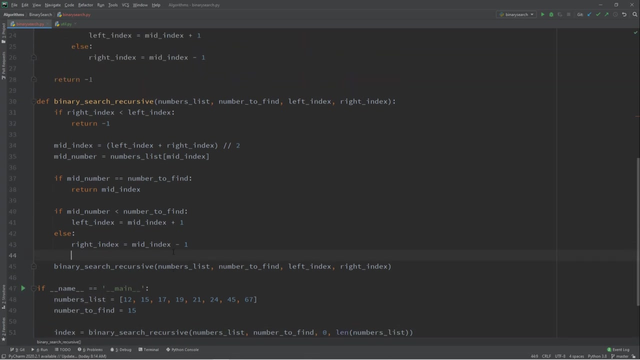 left and right index. okay, you call this function again recursively. so in that you have number list, you have number to find, you have left and right index, okay, and when you call this function for the first time, of course your left index is zero. your right index is the length of numbers list. I hope this is making sense. 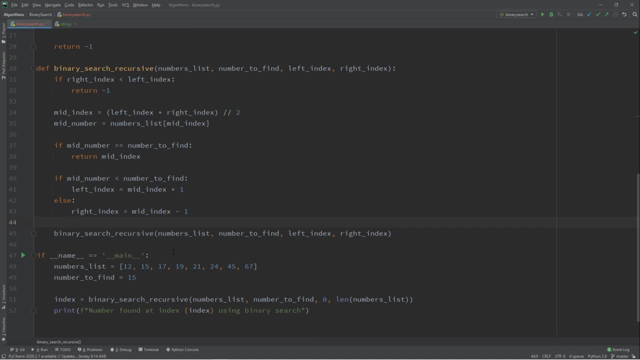 again, recursive function has no loops. the purpose of this function is to find your number in left and right index boundaries and if you don't find it, you reset your left and right index and you call this function recursively again. and by the way, when this function returns, 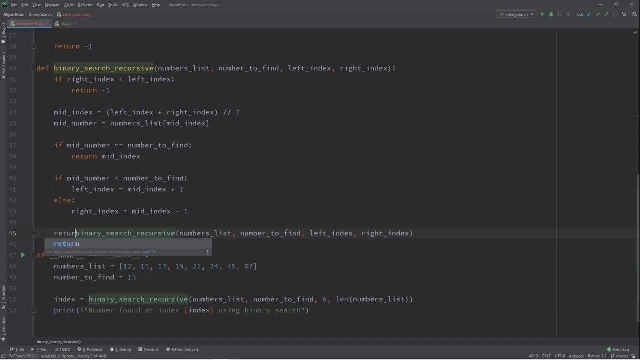 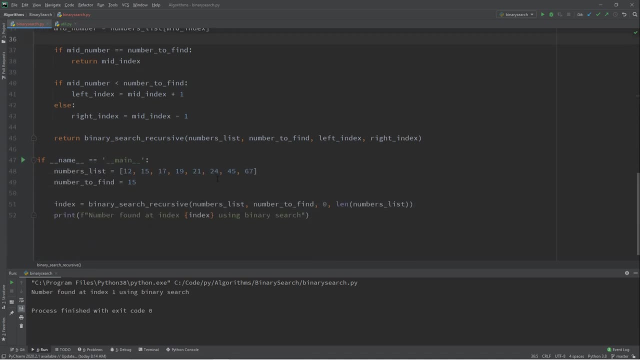 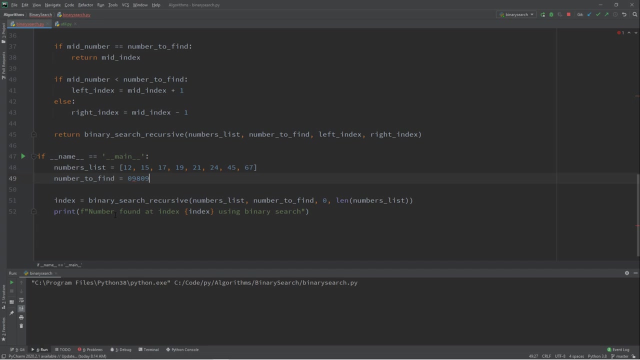 mid index. at some point you need to return that back. that's why this return statement is important. okay, right-click, run, see. we found 15 at index 1, so let's try to find 67. now see 7, and if you have random big numbers, it will return minus. 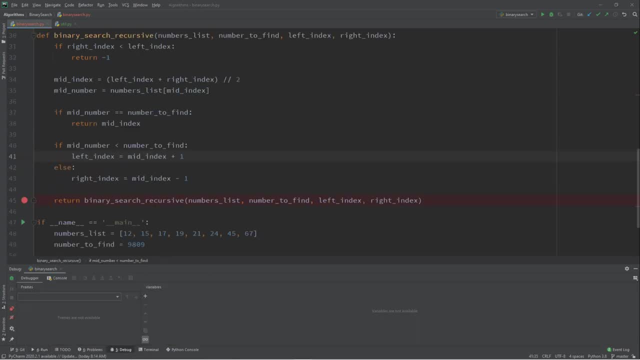 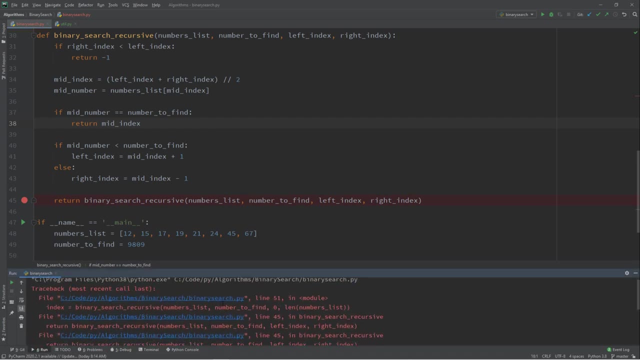 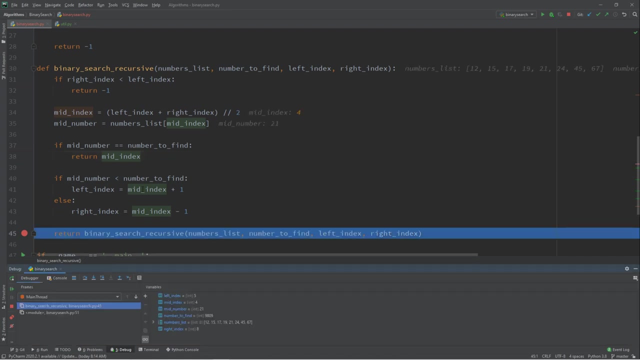 1. okay, so looks like when I run this I'm getting an error, because if you debug it, I try to debug it, and what I found was: let's see. so when I debug this, I keep on debugging this and at some point my mid index comes to be seven, and then that's. 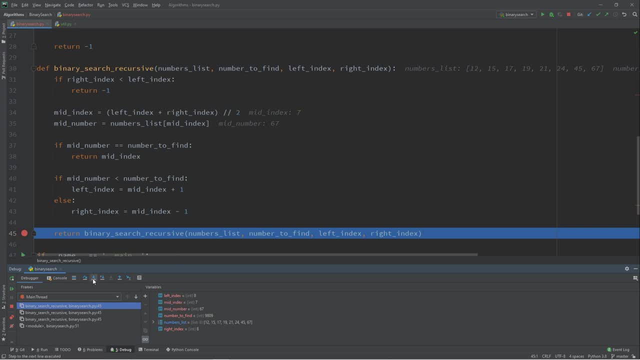 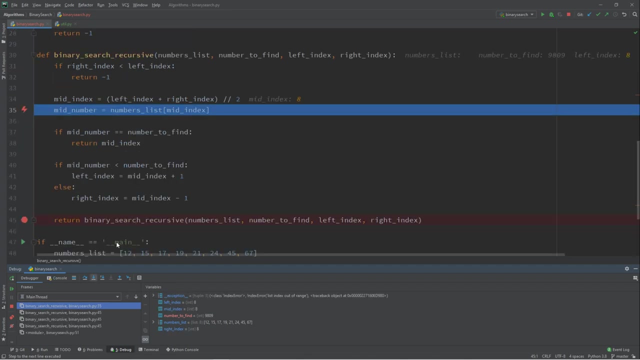 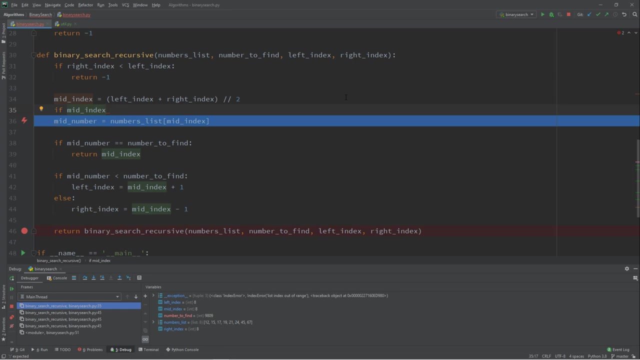 number 67. so let's say I'm at number 67 and when I go ahead, let's see. see, my mid index came out to be 8. so I want to check for my mid index here. so what I would do is, if mid index is greater than, let's say, length of number, 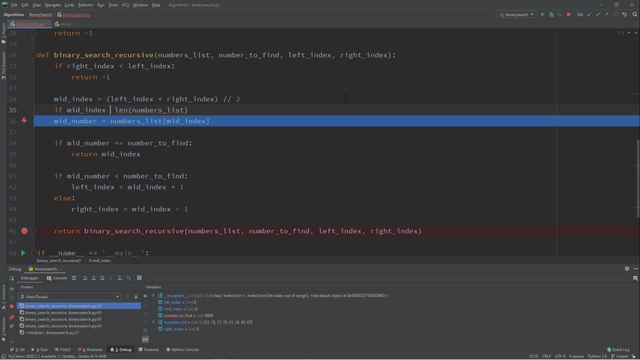 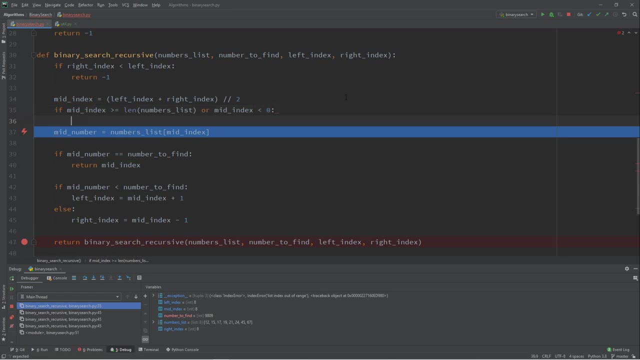 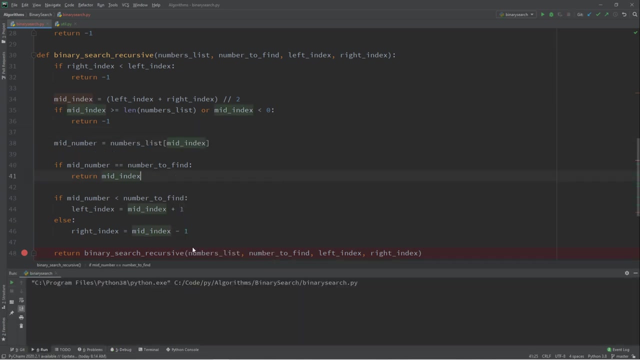 slits, or if it is equal to, greater than equal to or mid index is less than 0 due to some reason, return minus 1. this way your program is kind of safe, right, okay. and when you run it- see now it says minus 1, okay. so let's just quickly test. 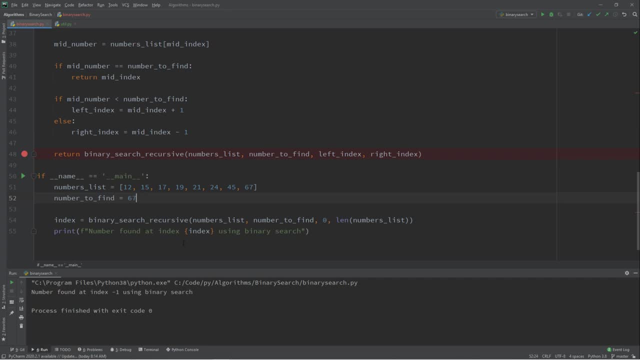 all corner cases. so in order to write good program, you need to taste all the different corner cases. which is last element, which is 7, the first element, which is 12, so it's 0. I will check any intermediate element as well, and all of that is working. okay, that's all I had. and now 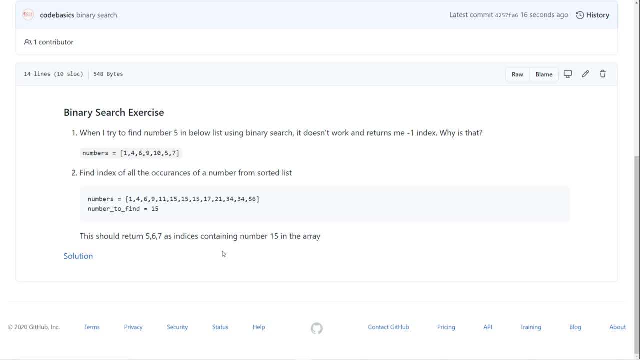 come back to the program and I will see you in the next video the most interesting part of this tutorial, which is an exercise. I have this two exercises for you and you need to solve these on your own before you click on the solution link, because the solution link has very bad virus embedded. 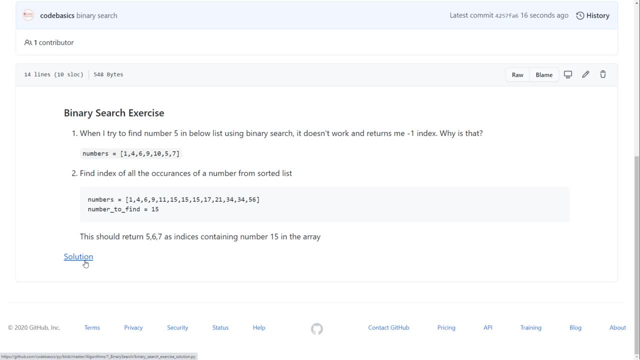 into it. so if you try to click on it before you try on your own, your computer is going to crash. so be careful. you do some coding practice on your own and then you look at the solution. data structures and algorithms are very, very important if you want to become a good programmer, so you cannot take a 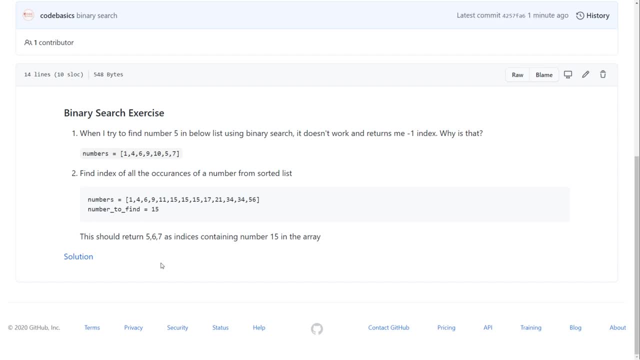 shortcut. you have to practice and make these concepts clear in your brain, doesn't matter which programming language you are using- Python, Java, Lara, well up, JavaScript, whatever the data structure and algorithms are everywhere, and the sound understanding of these concepts makes you a better programmer. I hope you liked this video. if you did, please give it a.